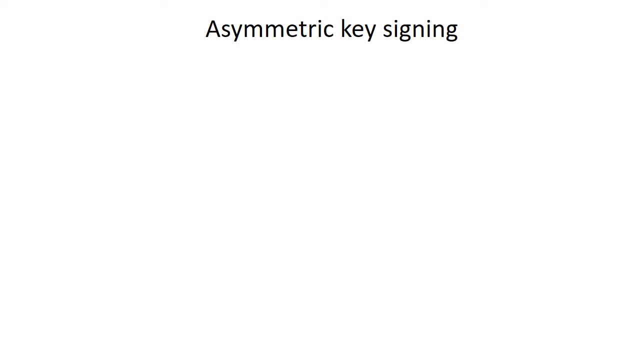 Asymmetric keys could be also used for signing the data, But in this case the data flow is opposite: The data sent from the owner of the key pair with the private and public key to anyone else. To achieve this, you want to want a receiver of this data to be 100% sure that this data was received from the owner. 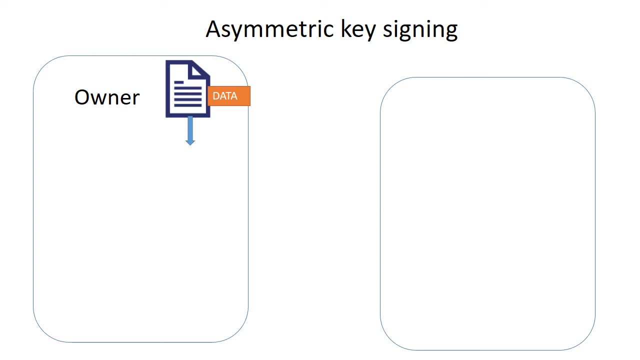 It means that no one else could send the same data, So this process is a two step process, Actually. the owner of the private key takes the data and create a hash of this data, And here we could use any hash function that we used or discussed before. Each hash will be unique and it will be a fixed length. 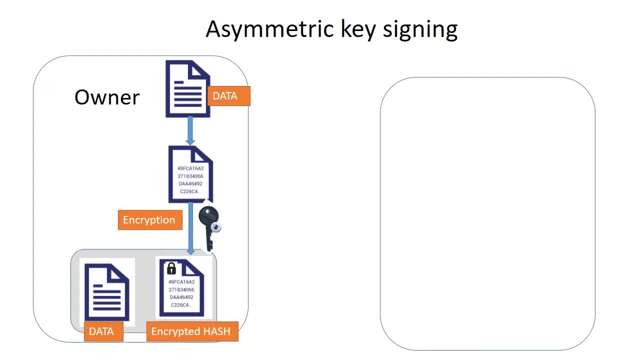 The hash is often encrypted using private key. The recap: We know that private key is only available for the owner, Nobody else knows the scheme. And after that the encrypted hash, along with the data, is sent to the another party, And this another party must be sure that data was sent from the owner. 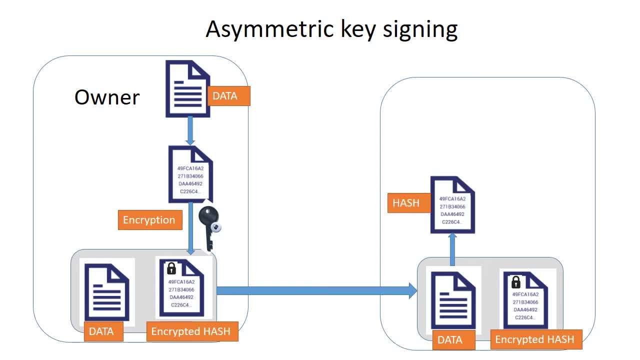 And that's why it verifies the data following way. It takes the same data using the same hash function, It create the hash. The data hash that was sent by the owner of the private key is decrypted using its public key And after that it compares those two hashes. 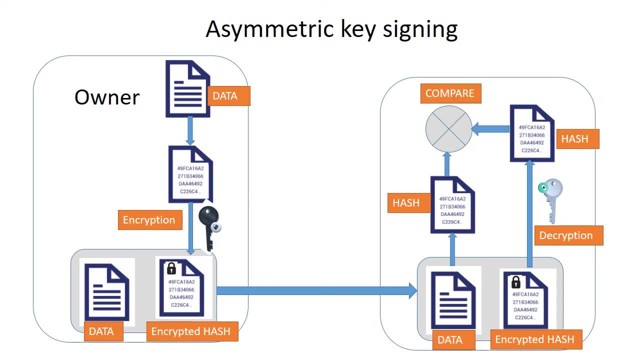 And if the hash match, then it is sure that the data was sent from the owner only. But you may ask what we achieve by signing the data using the symmetric key. There are couple of positive effects, So the first: in this case, we ensure that data was not changed during the transfer. 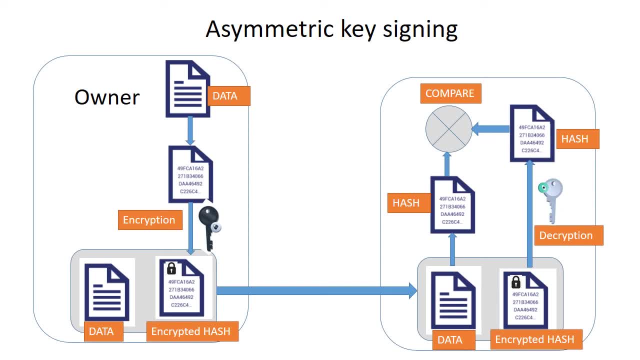 And second, if those hashes missed, we could be sure that data was sent, was sent exactly by the owner, And this part brought us is called a data signature. So in all the sense, the data using the private key- Actually it gets in fact- simply has created based on the date.